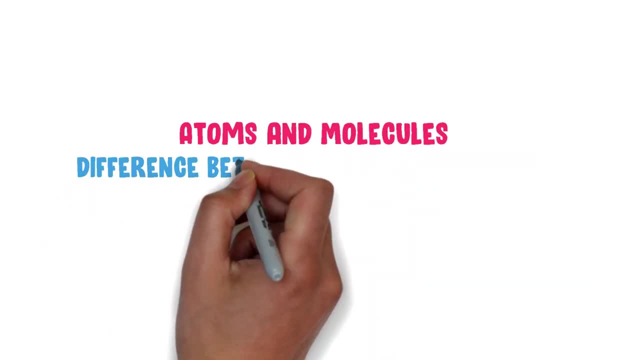 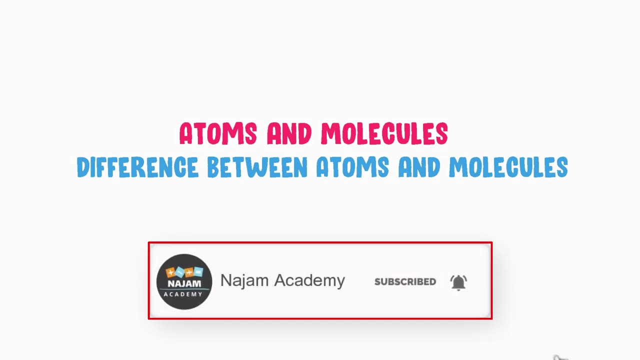 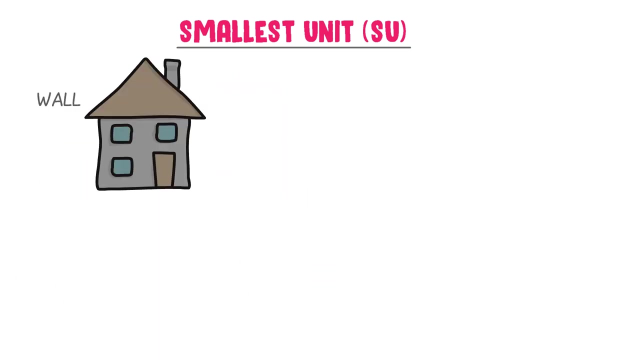 Atoms and Molecules. Difference between Atoms and Molecules. Before starting the lecture, click on the subscribe button and get access to our 100 of unique and simple lectures for free. Firstly, let me clear your concept about smallest unit, or SU. Well, consider a wall, a number 92 and a word: cat. 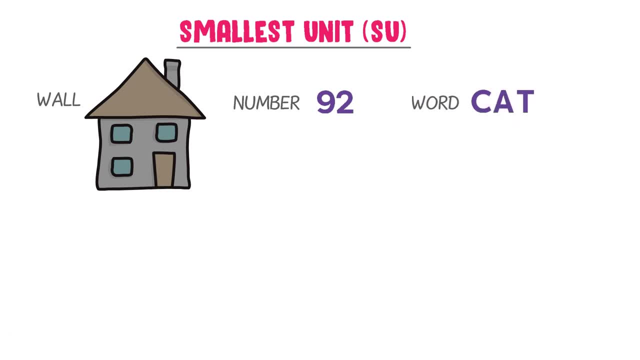 We know that the wall is formed by combining hundred or thousand of bricks. So brick is the smallest unit, SU or basic unit of the wall. Secondly, we know that 92 is formed from two digits, 9 and 2.. Here digit is the smallest unit- SU or basic unit of a number. 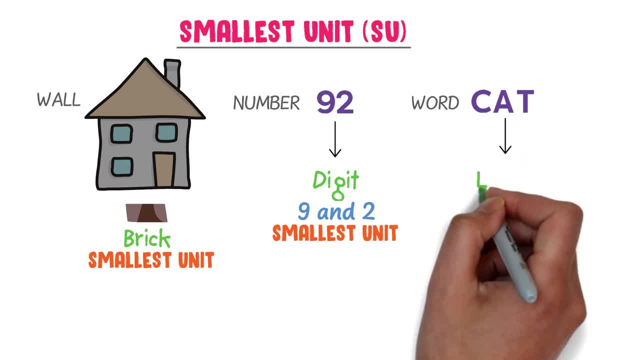 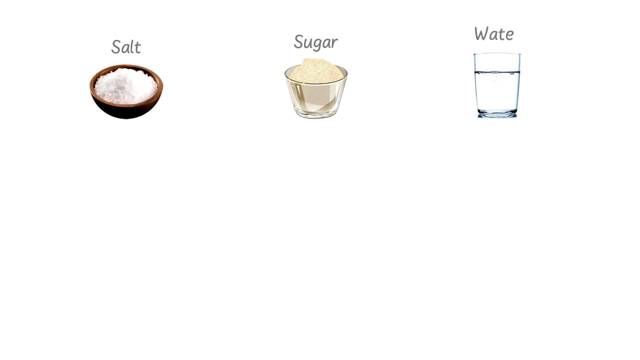 Thirdly, we know that the word cat is formed from three letters: C, A and T. So any letter is the smallest unit, SU, or basic unit of any word. Now consider salt, sugar and water. If we observe salt in electronic microscope, 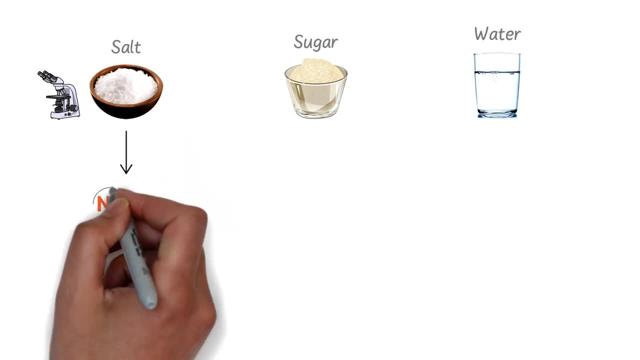 we see that salt is formed from two things: sodium and chlorine, And we cannot split up sodium or chlorine further. So sodium and chlorine are the two smallest units. SU are basic units of salt. Secondly, if we observe sugar, we get carbon hydrogen and oxygen. 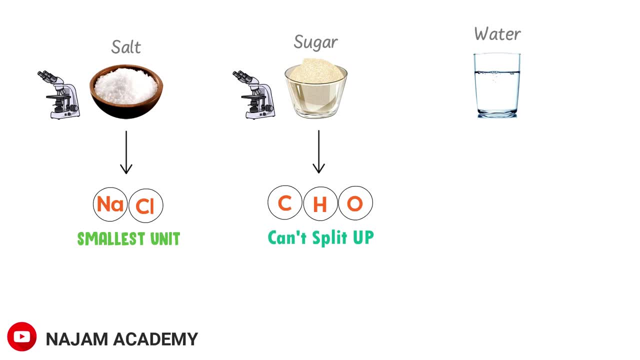 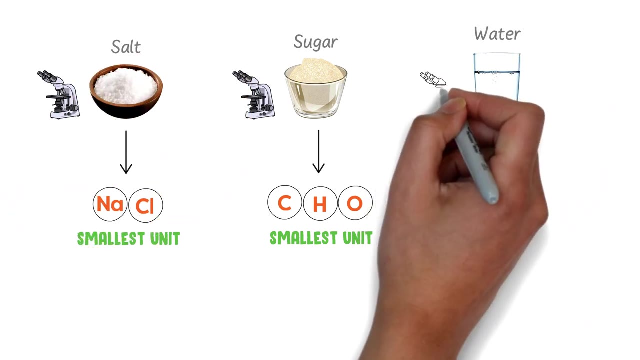 Also, we cannot split up carbon or hydrogen or oxygen further into something more simple. So carbon, hydrogen and oxygen are the three smallest units. SU are basic units of sugar. Thirdly, if we observe water, we see that water is formed from two digits, C and 2.. 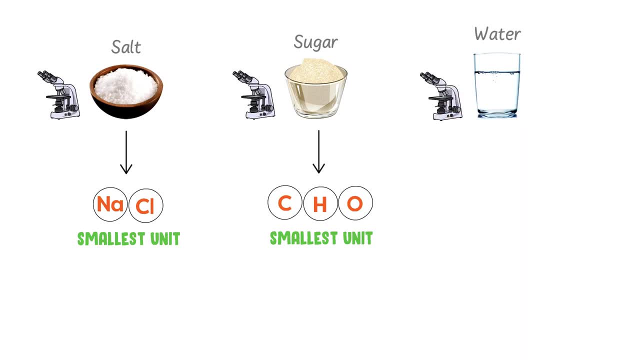 we observe water in the electronic microscope, we get that water is formed from hydrogen and oxygen and they cannot be split up further into simpler substances. So hydrogen and oxygen are the two smallest units, as you are, basic units of water. Now listen carefully, Brick. 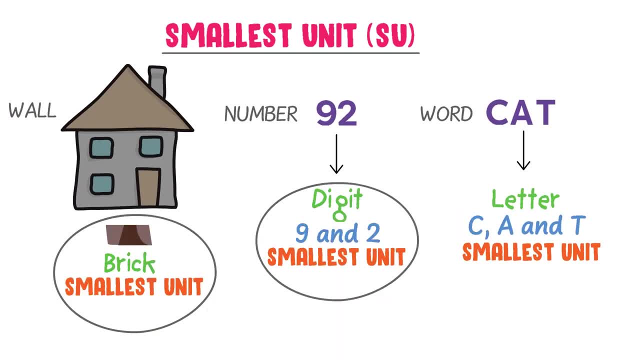 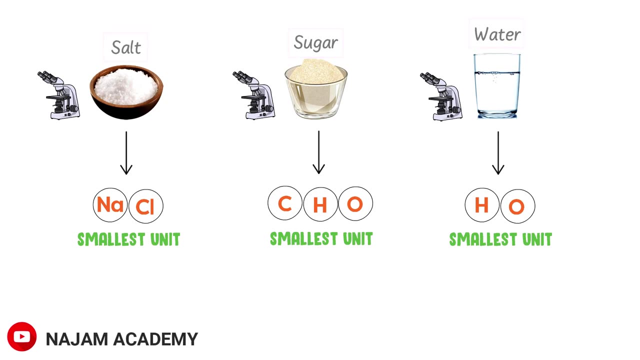 is the smallest unit of a wall. Digits like 2 or 9 is the smallest unit of any number. C, A or T is the smallest unit of any word. Secondly, we know that salt, sugar and water are all matter. So sodium or chlorine is the smallest unit of salt or matter, Carbon hydrogen. 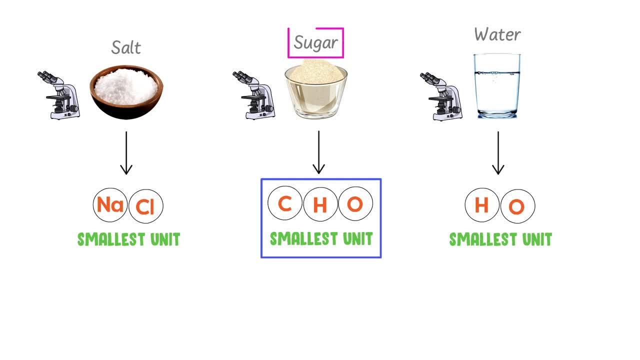 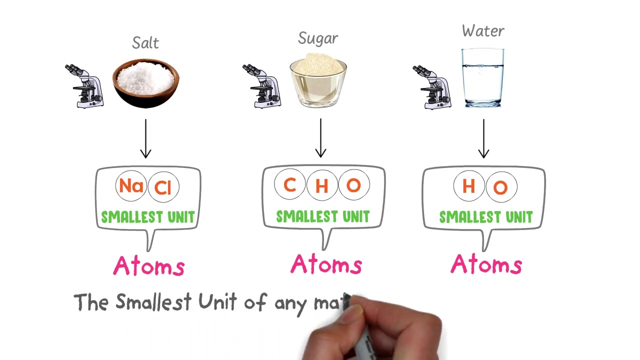 or oxygen is the smallest unit of sugar or matter. Hydrogen or oxygen is the smallest unit of water or matter. So these are the different smallest units of matter. In science we call these smallest units as atoms. Therefore we define an atom as the smallest unit of any matter is called an atom. 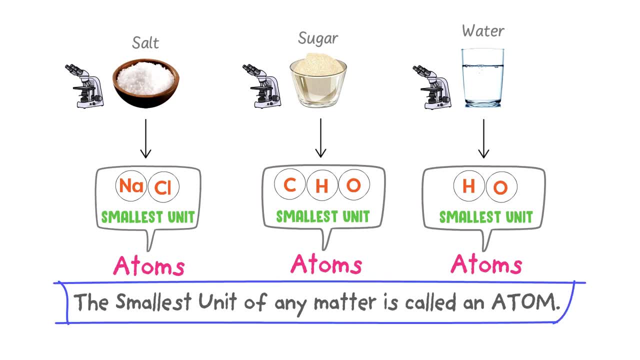 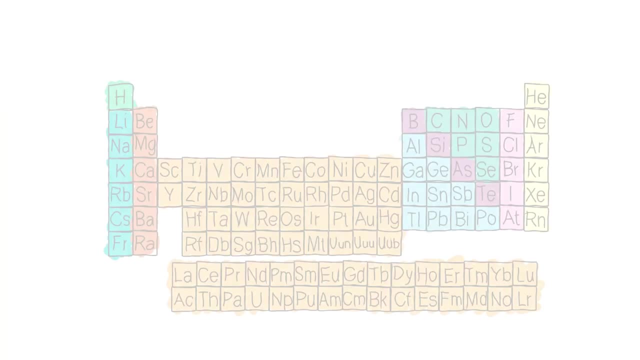 Let me repeat it: The smallest unit of any matter is called an atom. Remember that we cannot divide an atom further into something else. Now let me give you some examples of atoms. Well, consider a periodic table. We know that there are 118 elements in the periodic table. 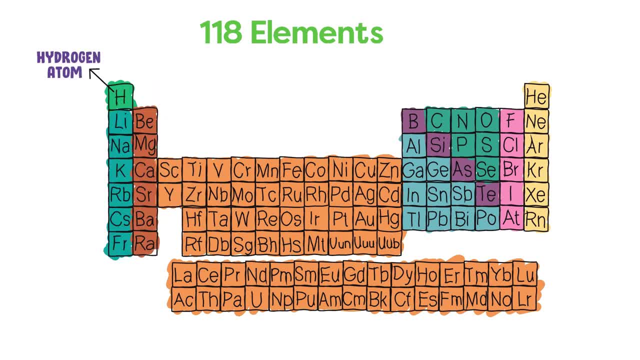 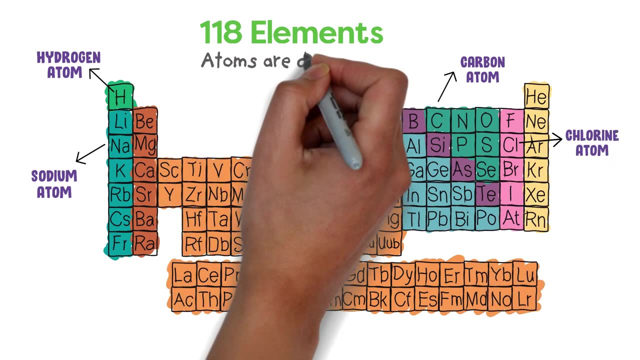 The smallest unit of hydrogen is hydrogen atom, The smallest unit of sodium is sodium atom, The smallest unit of carbon is carbon atom And the smallest unit of chlorine is chlorine atom. Also, remember that atoms are different from one another due to number of protons. 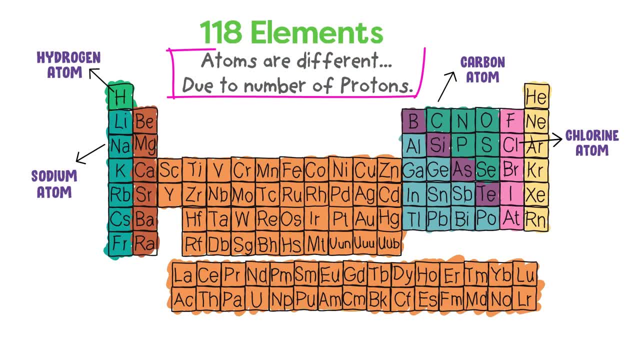 Let me repeat this important statement: Atoms are different from one another due to number of protons. For example, in the hydrogen atom, there is only one proton. In the sodium atom there are 11 protons, And the carbon atom. 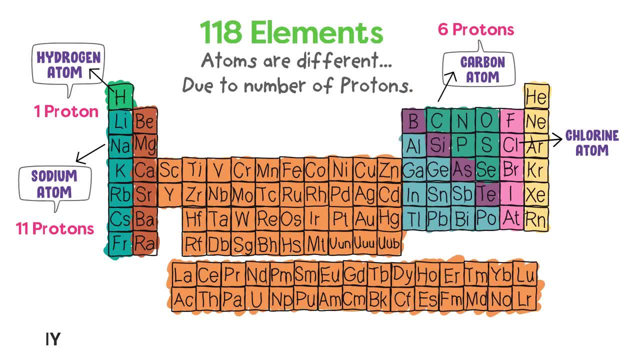 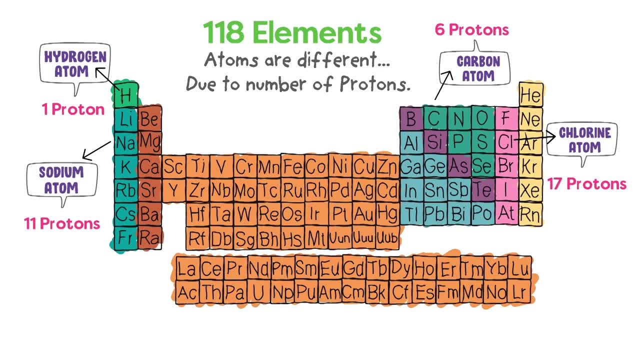 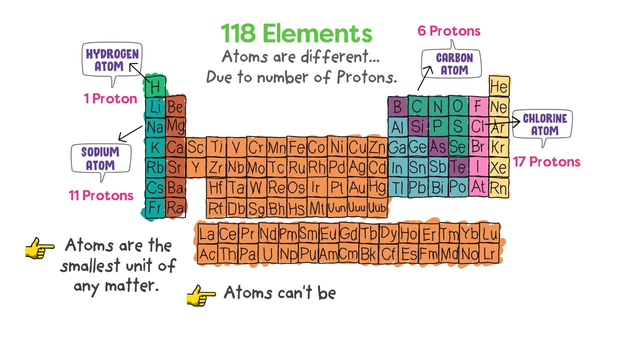 In the hydrogen atom there are 6 protons And in the chlorine atom there are 17 protons. Thus, remember these three important points about atom. Atoms are the smallest unit of any matter. Secondly, atoms cannot be divided further. 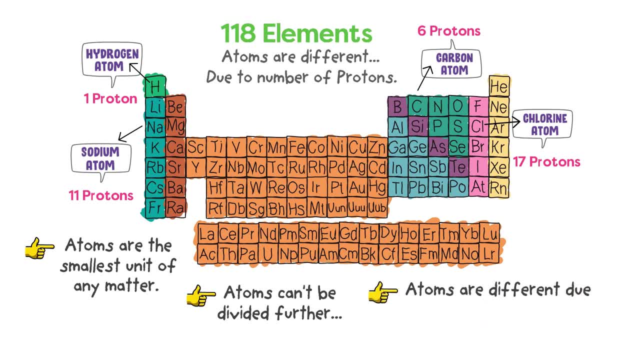 Thirdly, atoms are different from one another due to number of protons. Note it down, all these three important points about atoms. Note it down, all these three important points about atoms. Note it down, all these three important points about atoms. Now, what is a molecule? 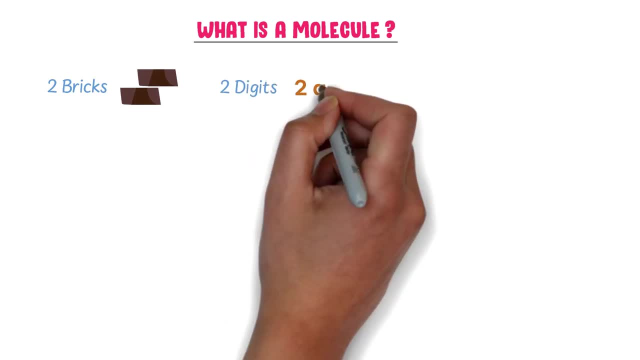 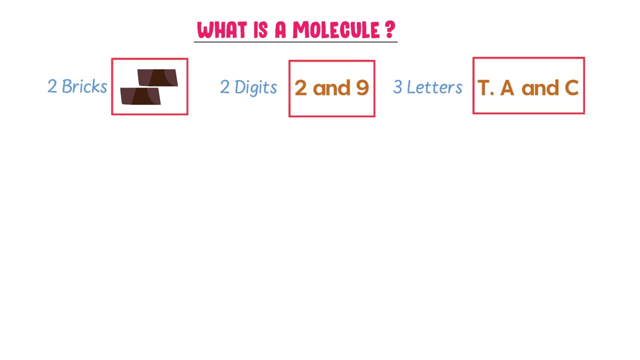 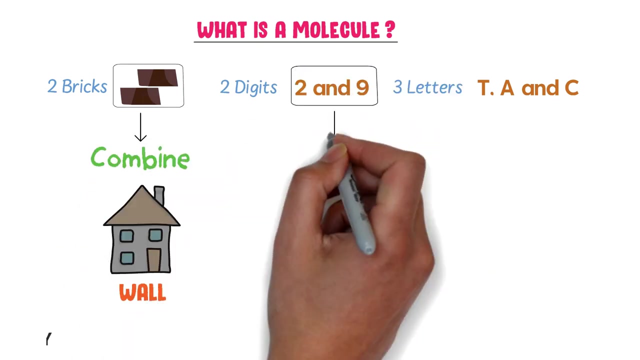 Well, consider two bricks, two digits 2 and 9, and three letters TAC. We know that these all are the different smallest units. Now, if I combine bricks, I get a wall. If I combine two digits- 9 and 2, I get a number 92.. 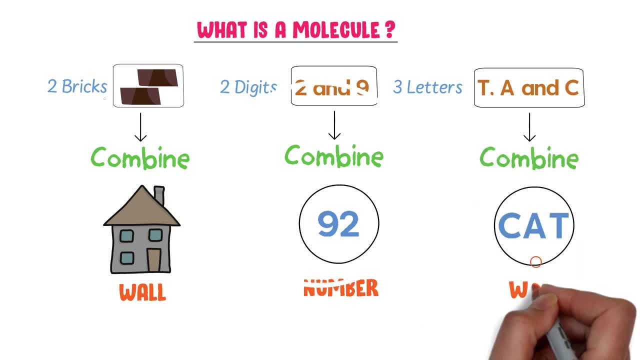 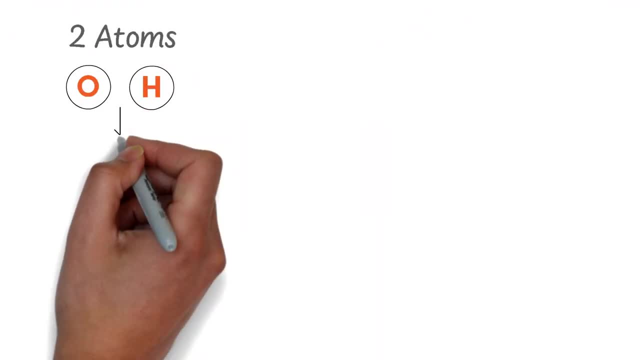 If I combine three letters C tässä, I get a word cat. Similarly, consider two atoms: oxygen and hydrogen. If I combine two atoms, I get a molecule of water, H2O. Consider three atoms: carbon, hydrogen and oxygen. If I combine, 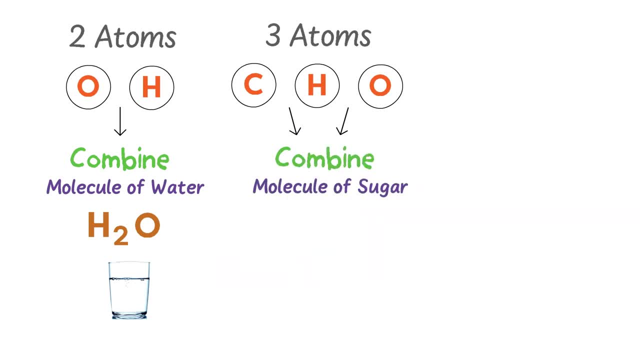 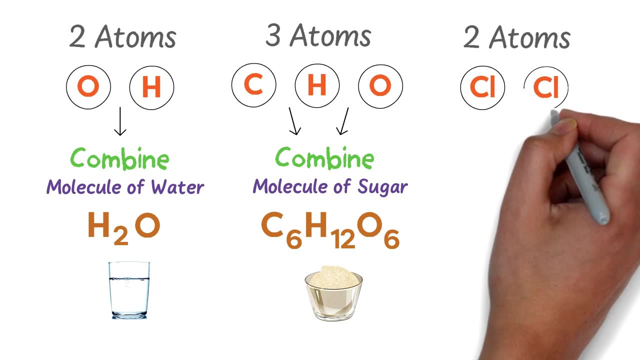 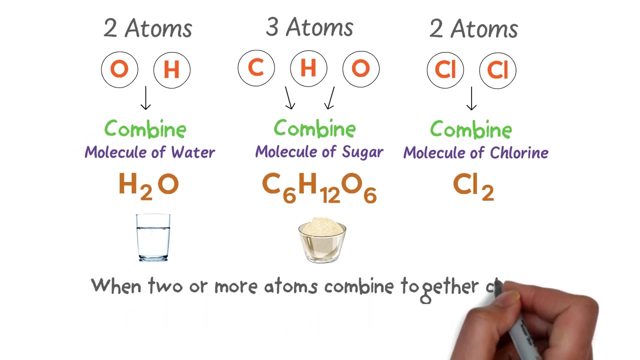 these three atoms, I get a molecule of sugar, C6H12O6.. Consider two atoms of chlorine and chlorine. If I combine these two atoms of chlorine, I get a molecule of chlorine gas, Cl2.. Therefore we define a molecule as when two or more atoms combine together chemically. 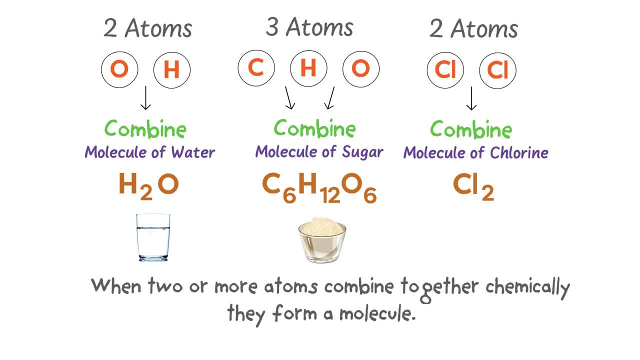 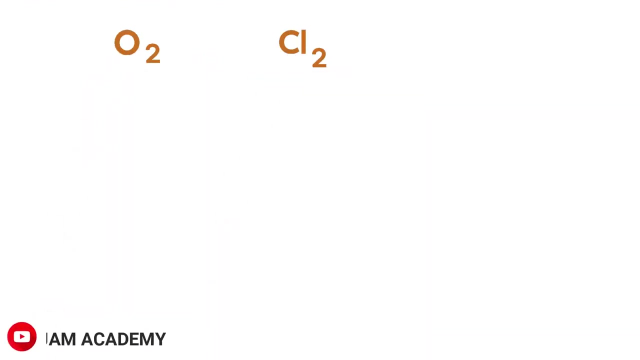 they form a molecule. Let me repeat it: When two or more atoms combine together chemically, they form a molecule. Thus, remember that when two or more atoms combine together chemically, we get a molecule. Also, let me give you some examples of molecules Like oxygen gas, chlorine gas, carbon dioxide gas, HCl or hydrochloric. 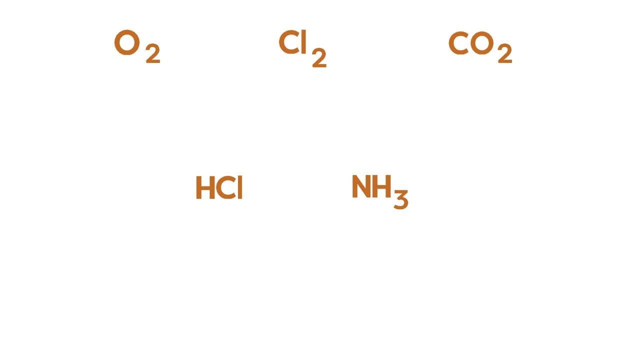 acid, NH3 or ammonia, etc. And And, And, And, And And. O2 gas. there are two atoms of oxygen, So it is a molecule of oxygen gas. And chlorine gas. there are also two atoms of chlorine, So it is a molecule of chlorine gas. 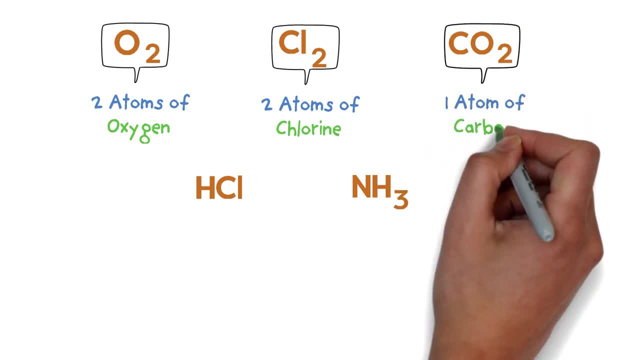 And carbon dioxide gas. there is one atom of carbon and two atoms of oxygen, So it is a molecule of carbon dioxide gas And HCl. there is one atom of hydrogen and one atom of oxygen And HCl. there is one atom of hydrogen and one atom of hydrogen, So it is a molecule of hydrochloric acid.